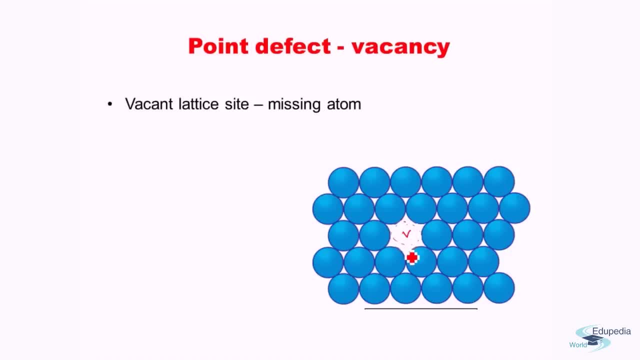 vacancy. So this is my vacancy Right Now. why is it that there is vacancy present? Why is it that all the lattice sites are not occupied by atoms? This is so because thermodynamically, it is impossible to create a vacancy free solid. Whenever the temperature is greater than zero, Kelvin temperature is 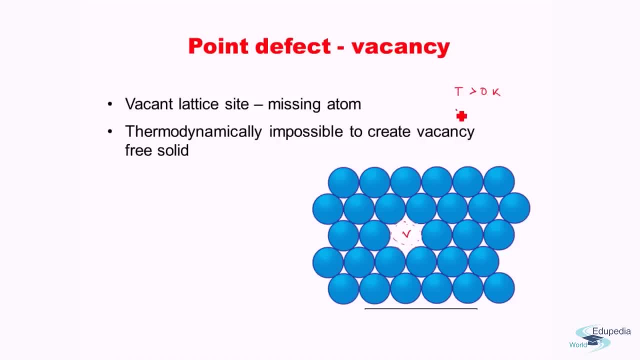 greater than zero Kelvin, Vacancy will be present. Vacancy will be present. It is impossible to have a vacancy free, solid, at temperature greater than zero Kelvin. Now, what is the expression that will give you the relation between temperature and vacancy? So basically, 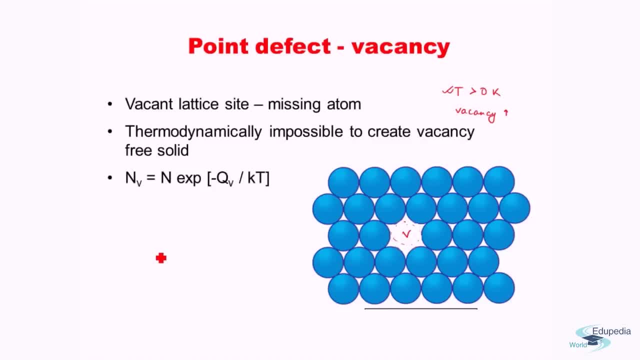 this relation gives you idea about how many vacancy. what is the amount of vacancy that will be present in a crystalline material? let me define the terms. NV is that total number of vacancies that will be present in a thermodynamic state. n is the total number of lattice site right. 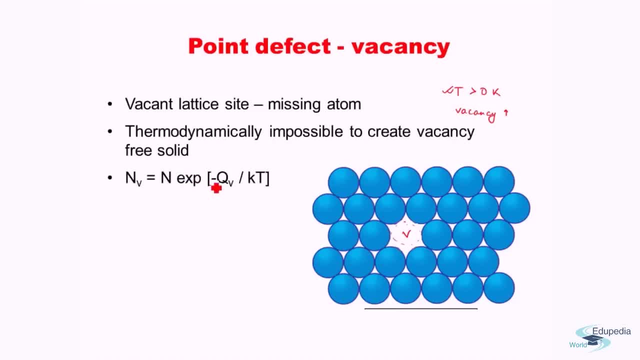 and exponential minus QV by KT. QV is the activation energy for vacancy, so how much energy is required to form a vacancy? K is basically the Boltzmann constant and T is temperature in Kelvin. okay, so if we try to realize what exactly this equation says, this equation is in e to the power minus Q by KT. so 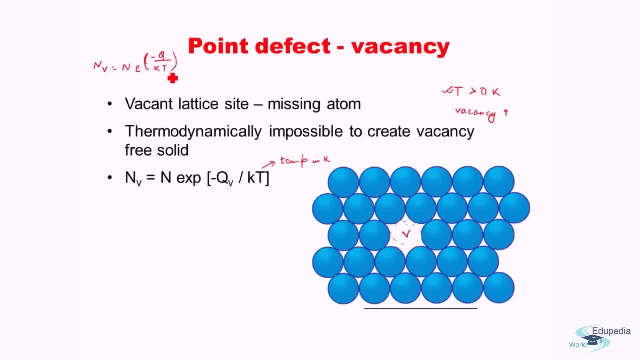 here we see that if we increase temperature, then this whole thing is going to increase. or this whole thing is going to increase because here it is in the denominator: it's going to increase, this is going to decrease, but this is negative, so the whole thing is increasing. 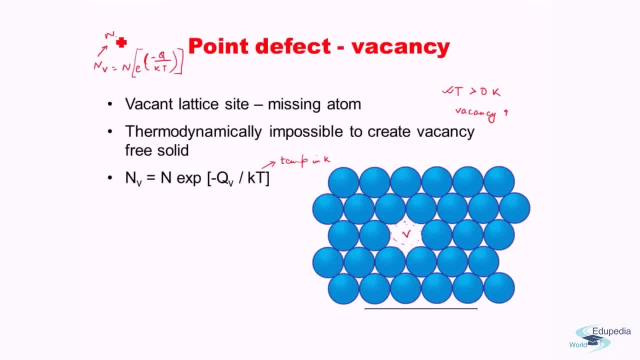 thereby, number of vacancies increases as temperature increases. okay, and we can also see from here that the amount of energy required to create a single vacancy, if it is high, then the number of vacancies will be low, and this thermodynamic equation is exact reason why we cannot create a vacancy free. 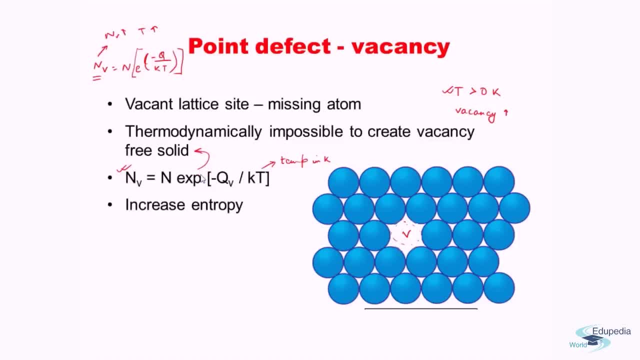 solid. okay, we now know that the thermodynamically it is not possible to create a vacancy free solid, but the basic idea is that the presence of vacancies is increasing the entropy of the system, and the exact number of vacancies which will have maximum entropy will be defined by this. so we know that the universe tends towards increasing the. 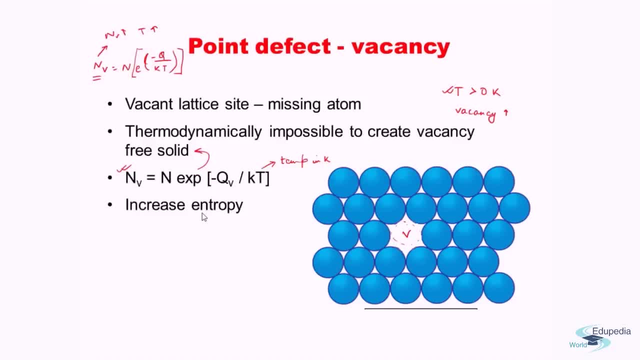 entropy. so this is the reason: the increased entropy is the reason for presence of vacancies. fine, and, as I already mentioned, higher the temperature, more will the number of vacancies, as given by this equation. so we now understand that vacancies are a very important and integral type of point defect which will more or less 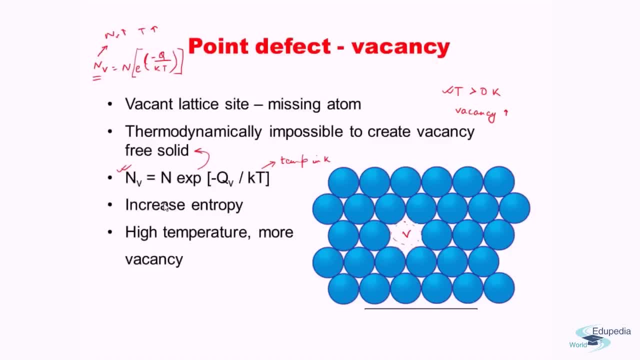 always be present. the only condition it might not be present when we have absolute zero temperature, which is not achievable. okay, so now you will ask me: what is the importance of vacancies? the importance of vacancy, as we'll see and understand in the later processes, is that it helps in diffusion, right? if imagine there was a atom here too, all the atoms were in the 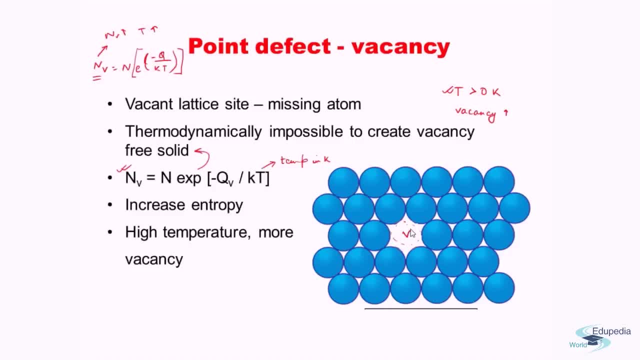 location where they were supposed to be, then any atom cannot travel from here to here. you have to break all the bonds, then the atom will have will be able to travel somehow, right, but if you have a vacancy here, then this atom, this atom can jump here, okay, and 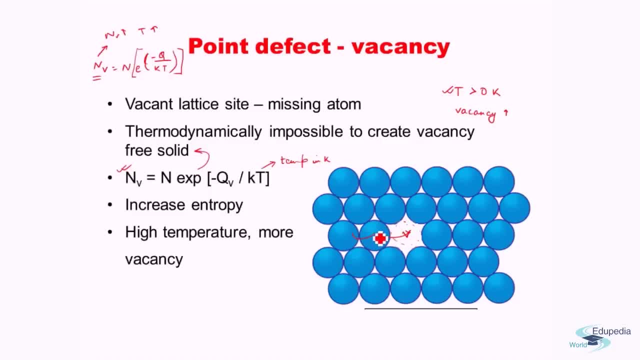 the vacancy, as a result, comes here, then this atom can jump here and the vacancy comes here as a result. thereby the vacancy travels one way and resultant atom travels the other way. now just imagine that you have so many vacancies, a large number of vacancies, right, and as a 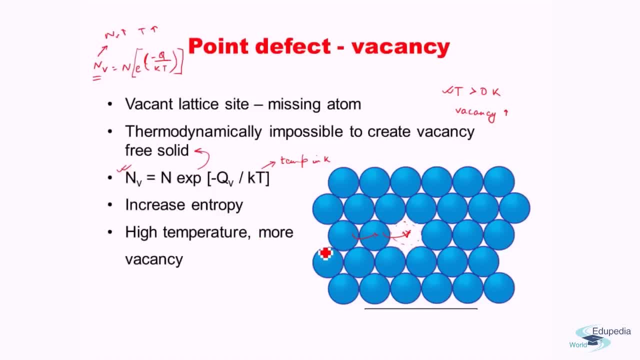 result, what can happen? the atoms will be free to diffuse through the material, and this idea that diffusion can take place due to the presence of vacancies is kind of a pivotal idea in defining the properties of the material. we will understand that when in our future lectures. next let us see the second kind of point- defect in metals- which is self-interstitial. so here 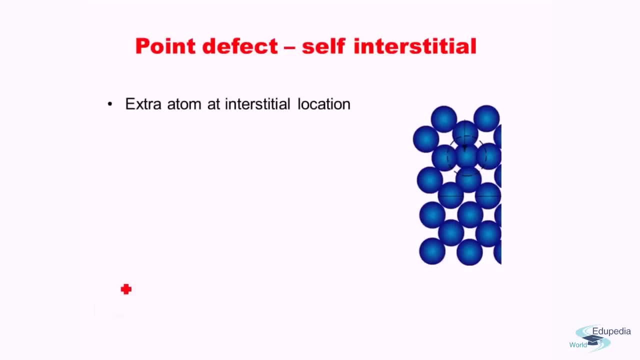 i have shown you the idea of self-interstitial. as the name suggests, self-interstitial means the same atom type is additionally fit into the interstitial void, so ideally atoms should have been at these locations. right, it should not have been here, but a atom is fit over here to an additional. 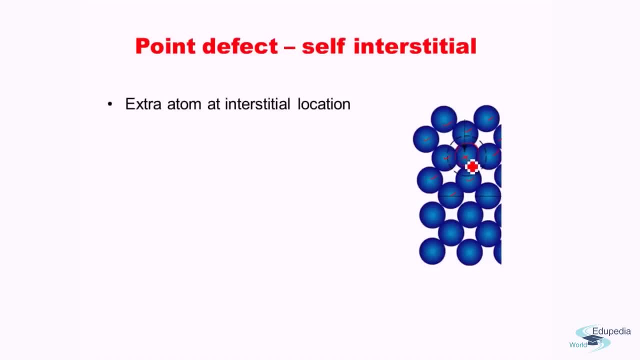 atom, that is to say, and this extra atom is what is basically self-interstitial- self because it is. it belongs to the same metal type as the metal which is made up of the same metal type. same if these are iron, then this is also iron and interstitial because it is. 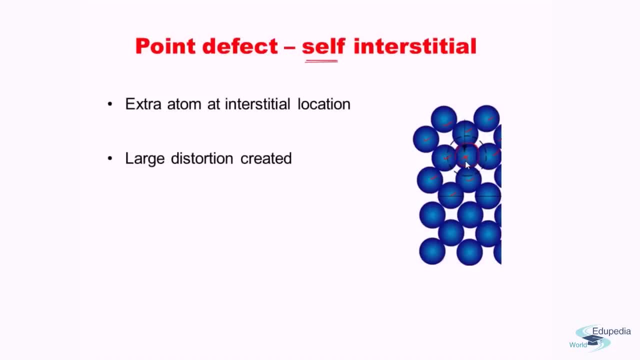 in the interstitial void location. but as you see that since it is the same metal type or the same element type, the sizes are same, but we know that the interstitial voids are quite small compared to the atomic size. therefore, in order to accommodate this additional atom, the surrounding atoms will have to 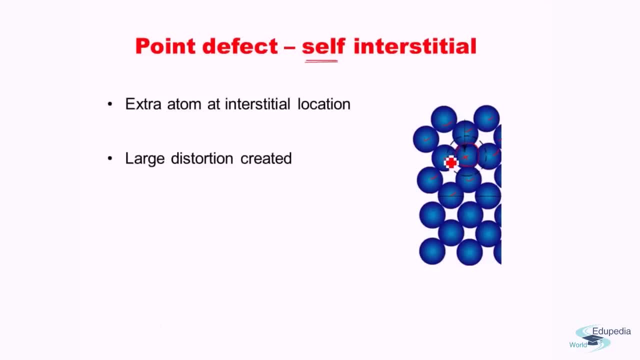 be kind of pushed away. this atom needs to move away. this atom needs to. all the surrounding atoms need to move away, and this atom moving away will create movement of the further surrounding atoms right. thereby a large distortion is created in the vicinity of the self interstitial. 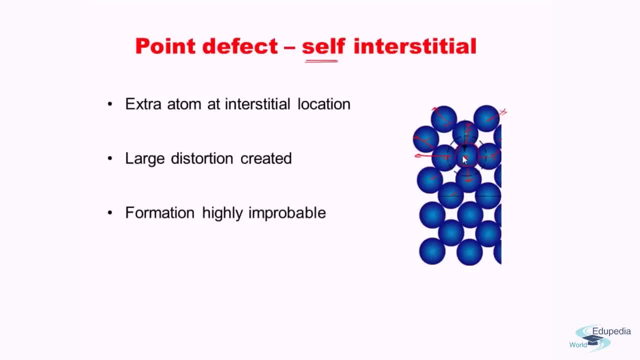 atom and due to this idea that a large amount of distortion is created, which means a large increase of energy is there? distortion is a result of energy enhancement. right, therefore, it is quite a improbable scenario to form self interstitials, that is to say, even if the 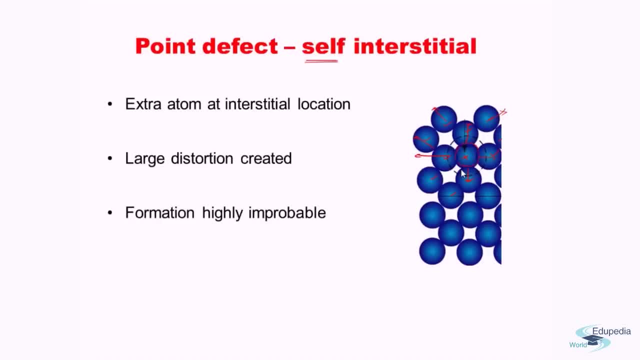 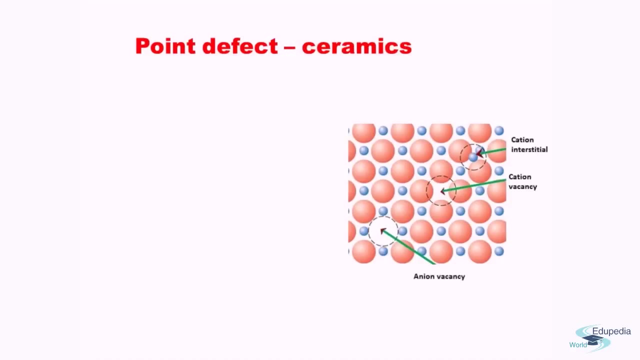 self interstitial atoms are present, they will be very less in number, okay, much, much less than vacancies. fine, now let us see the cases of ceramics point defects. in ceramics, as this image suggests, we can have different kind of point defects. what are those? we can have vacancies and we can have interstitial. 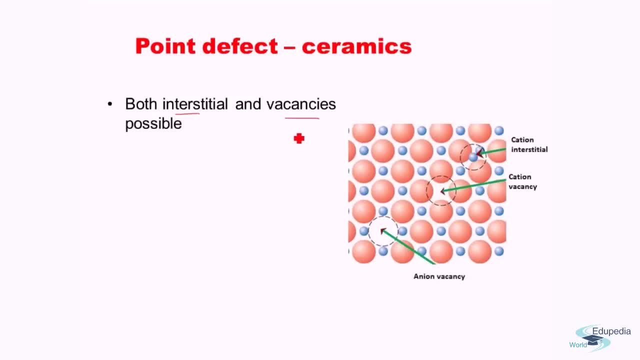 same as in the case of metals, but here the vacancies can be of two types. it can be an ionic vacancy or it can be a cationic vacancy. here we have shown the smaller atoms as cation and the larger atoms as anion. because that 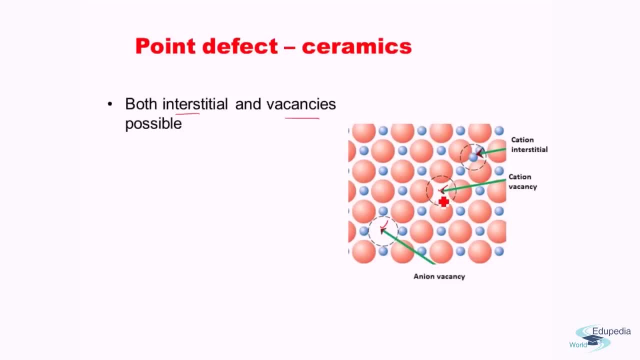 is normally the case. so we can have anionic vacancy, we can have cationic vacancy. in addition, we can have interstitials and the interstitial atoms will normally be cationic interstitial, because anionic interstitials will be very large and lot of distortion. therefore it is. 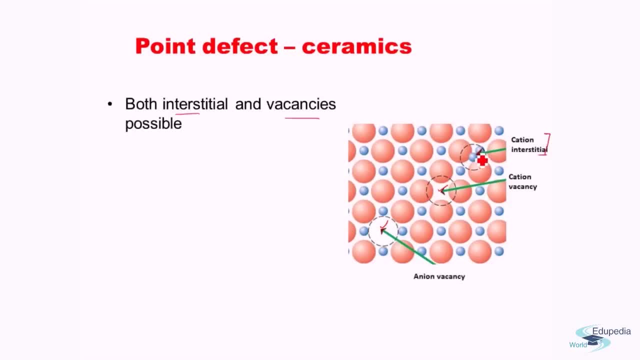 mostly improbable. we can have cationic interstitial because they are smaller in size and they can fit in the interstitial sites okay. and since we have more than one kind of atom, we have more, hence multiple kind of defect, as I have already shown here. and anion being large, anion interstitial is normally 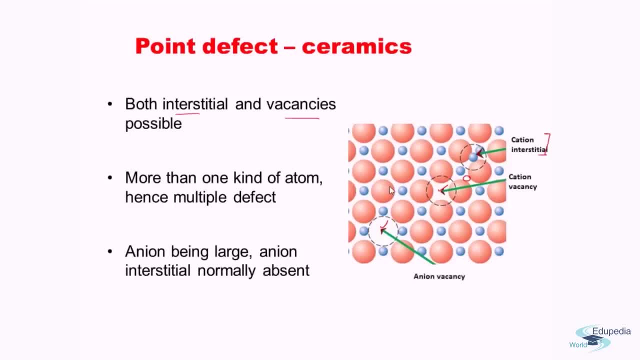 absent. so this concept over here. we have the following concept of cationic defect, as I have already shown here, and anion being large, anion interstitial, is normally absent. so this concept over here. the point defect for ceramics is parallel to the concept for metals. the 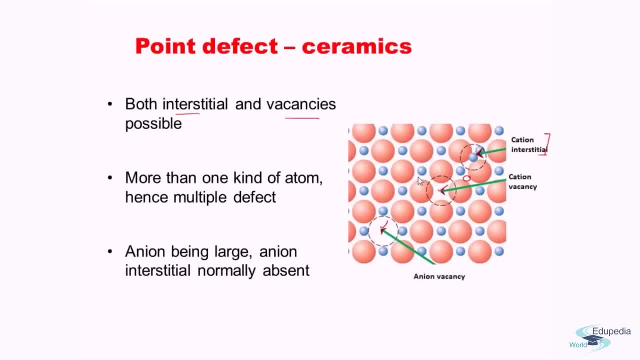 only difference is, since there is multiple types of atoms, there will be multiple types of defects parallel to the metal scenario. okay, now this combination of defects- point defects- basically gives rise to certain type of defects which are very typical of ceramics, and they are very important to the properties of ceramics too. to begin with, we will discuss about Frankel. 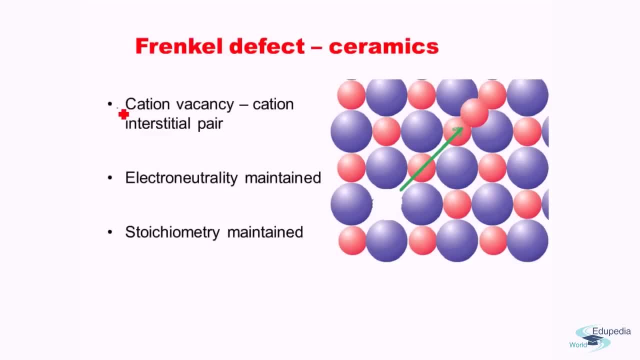 defect now Frankel defect- is basically a cation, vacancy anion interstitial pair. what do we mean by that? what we mean is: here there was supposed to be a cation, right, the cation was supposed to be a cation and the cation was supposed to be a. 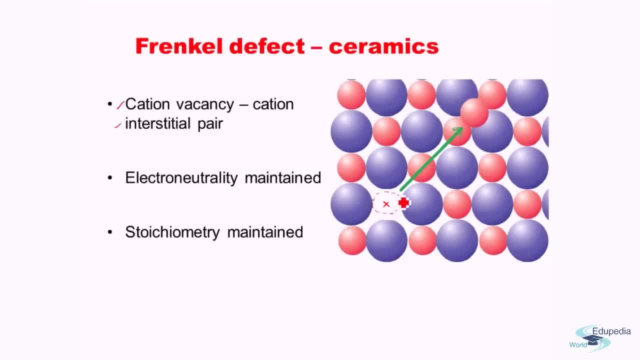 supposed to be here, which is not there, so it is absent. but this cation has basically been displaced from here to a interstitial site. okay, so it has traveled from here to there and now it is at the interstitial side, so we have a cation. 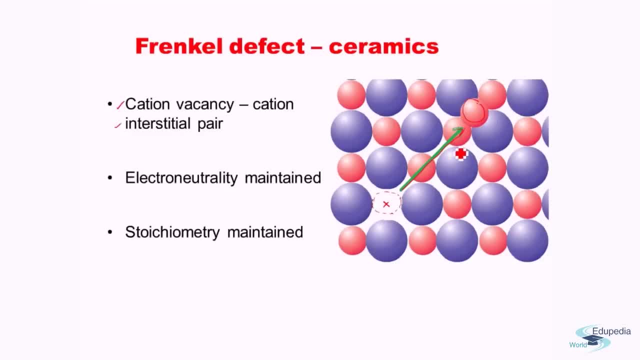 vacancy and a cation interstitial, and this exists in pair right now. why do they need to exist in pair? they need to exist in pair. they need to exist in pair because they need to exist in pair because the electrical neutrality needs to be maintained. what do I mean? the idea. 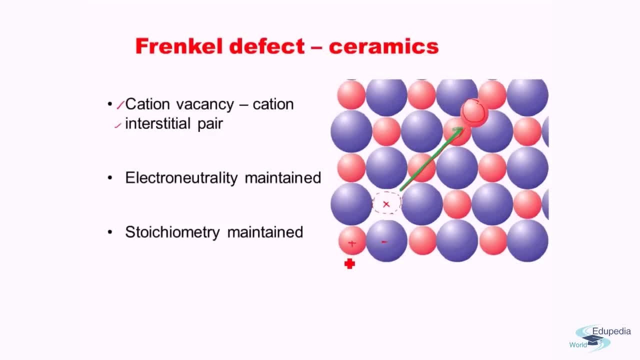 is that this being an anion will have a negative charge. this being a cation will have a positive charge. now suppose I just removed this cation from here right? thereby I am removing a positive charge. the whole material will gain a negative charge. thereby the electrical neutrality is not maintained. therefore the cation cannot. 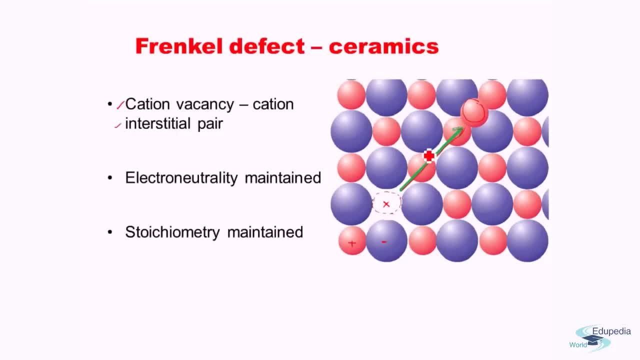 just leave the material. it can leave the leave its location and go to a different location whereby the electrical neutrality is maintained. okay, so electro neutrality is the prime concept when discussing with defects of ceramics. it, the whole material should be electrically neutral. fine, and also, here we see, the stoichiometry is maintained. why? because one cation is lost. 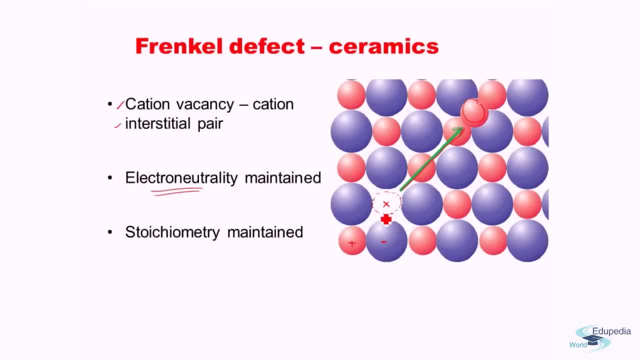 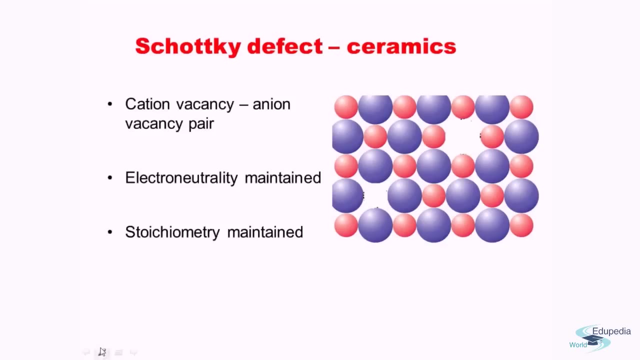 but the same cation is gained at a different location. thereby the whole stoichiometry is maintained. so this cation, vacancy cation, interstitial pair, this is what is known as a Frenkel defect. okay, next let us see what is a Schottky defect. so 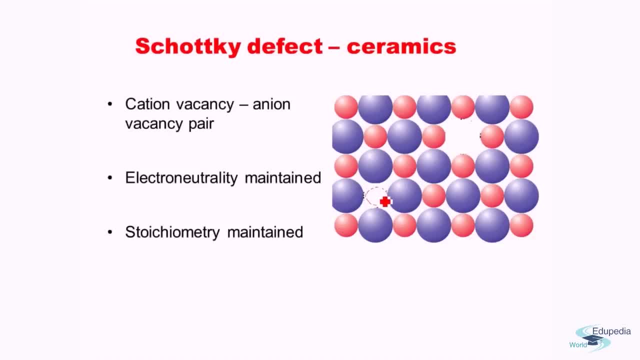 So a Schottky defect is a little different than Frankel defect in that we have a missing cation, same as a Frankel defect, but this cation is completely missing from the specimen. and to counteract this, that is, to undo for the charge loss, we also miss a anion right. so 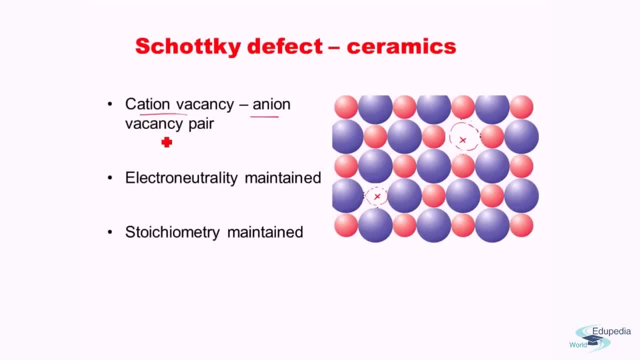 we have a cation missing and we have anion missing. that is what is Schottky defect. is cation vacancy, anion vacancy pair is Schottky defect and electrical neutrality is maintained in this manner right that both are missing so as to maintain the electrical neutrality. 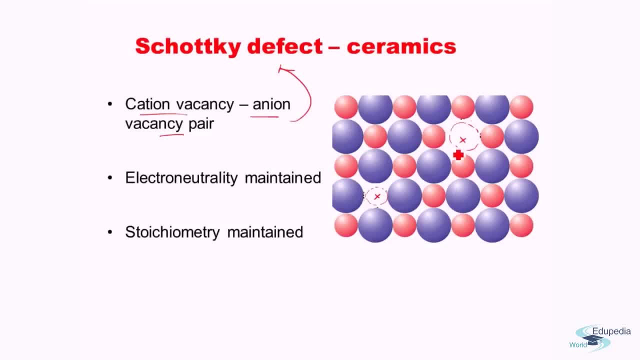 and also the stoichiometry is maintained. how come? because the ratio in which the cations and anions are missing is in the same ratio as their stoichiometry, so as to maintain the electrical neutrality. Okay, So this gives you an idea about the kind of point defects that exist in a ceramic mostly. 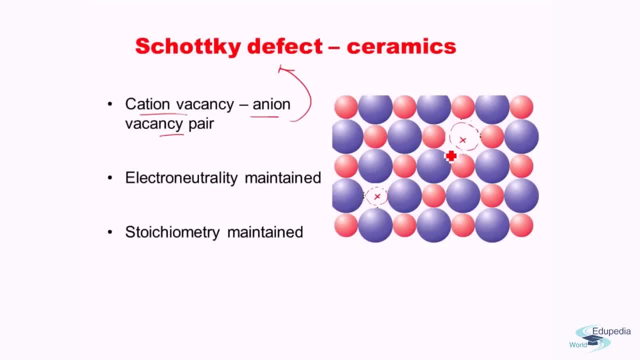 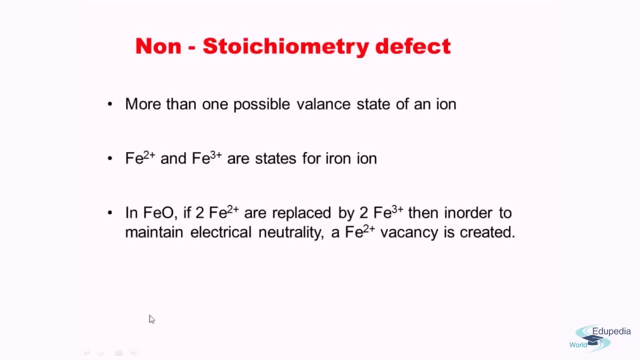 they exist in pairs. Next up I will discuss a different kind of point: defect in ceramics which can exist individually too, that is, non stoichiometric defect. Suppose you have a ceramic which can exist in more than one possible state or more than one possible. 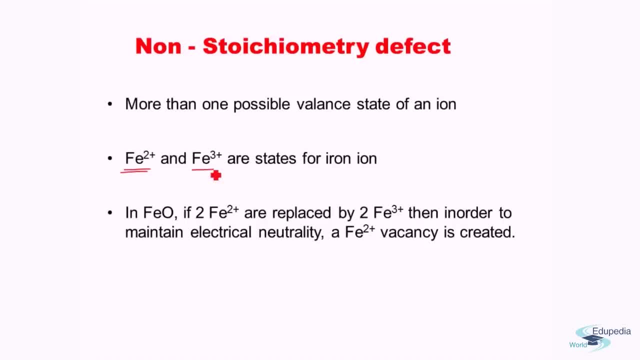 Like an ion. we know that ion exist as 2 plus as well as 3 plus right now, if I have Fe O right. so Fe O is basically Fe 2 plus and O 2 minus. now suppose that I replace 2Fe 2 plus. 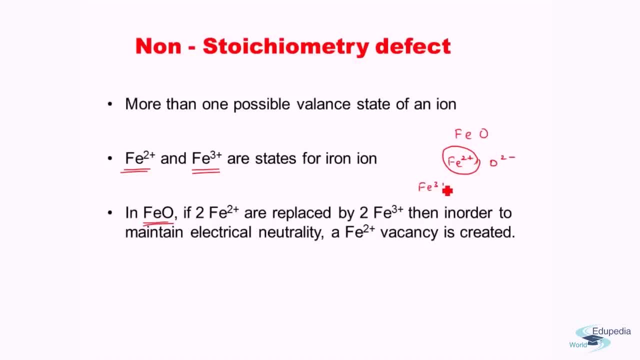 I replace 2Fe 2 plus by 2Fe 3 plus. Okay, So I replace Fe 2 plus by 2Fe 2 plus. so what will happen? two fe2 plus i am replacing by two fe3 plus, thereby additional plus two. 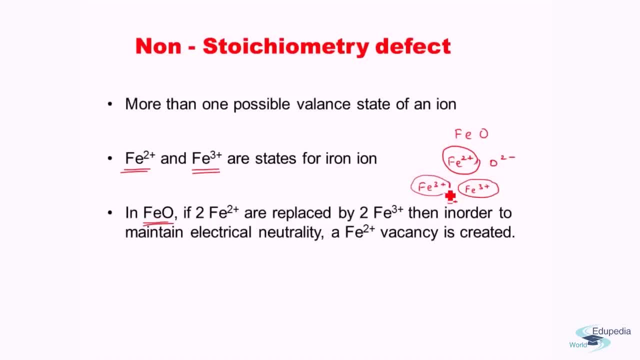 charges gained right, because one additional charge from here, one additional charge from here plus two charge effectively is gained. therefore, to maintain electrical neutrality, a fe2 plus needs to be missing- missing right: an additional fe2 plus needs to be missing. then that loss of two plus and this gain of two plus will be counteracted. 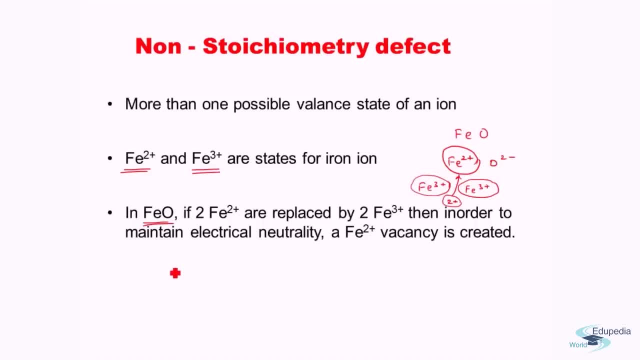 which means that in order to add two fe3 plus, we have to subtract three fe2 plus in order to maintain electrical neutrality. so what is happening here? so what is happening here? we are removing three things and we are putting two things right. we are removing three fe2 plus. 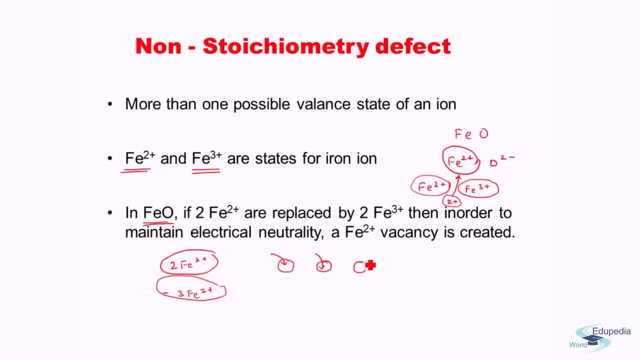 and we are just putting two fe3 plus, so we have a location where atom is missing, where there should have been an atom right. as a result, what we have is a vacancy here, but the electrical neutrality is not there. so we are removing three things. electrical neutrality is still maintained because of different possible valency state. 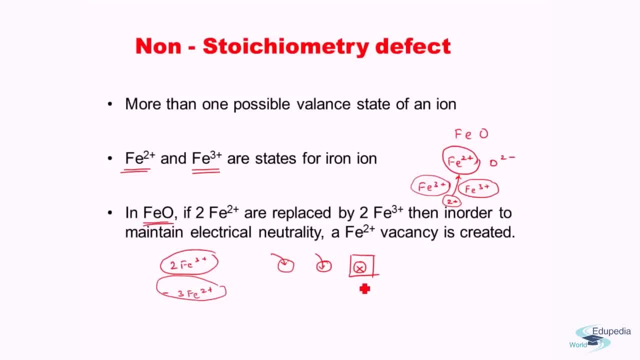 and this missing vacancy results in a non-stoichiometry right, because the ratio of fe is to oxygen is no more one is to one. now fe has reduced, it becomes something like 0.95 is to one. okay, and uh, this is what is non-stoichiometric defect. here we have our single defect. That is the. 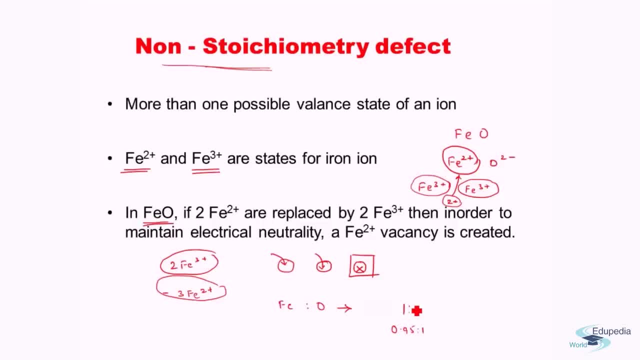 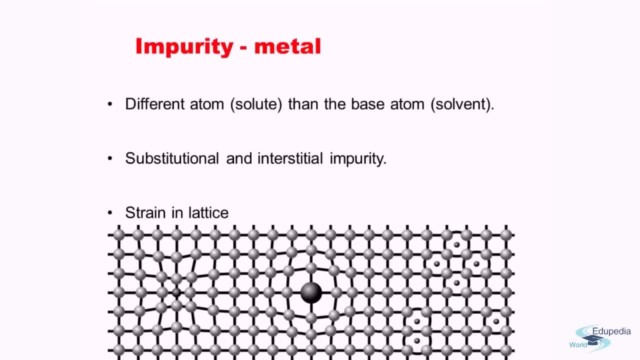 defect does not exist in pair, even in a ceramic system. Next, let's see the cases of impurity defects. First, in the case of metal. So, as I discussed, let us imagine iron and in Iron. In Iron, if we have a case of cursed metal. in case of this case, if we were to use a passive cheese, lährimahine squares to make IKEA and uh in iron to beucker case fonts, like on the material. who's considered, for example, iron or després, as well as iron layer, de in iron? it should not have multiple items of which probabaly should be in mark. here one is applying water. 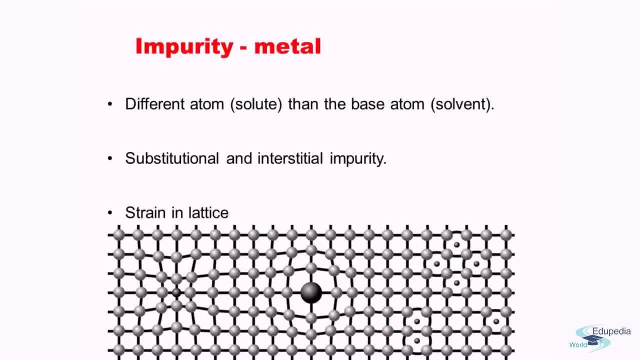 all the iron atoms are located in its lattice site, everything is fine and perfect. okay, now if i add carbon into it? fine, if i add carbon into it, then the carbon will go somewhere. carbon being much smaller than iron, it will go into the interstitial sites. okay, so if the impurity atom or the 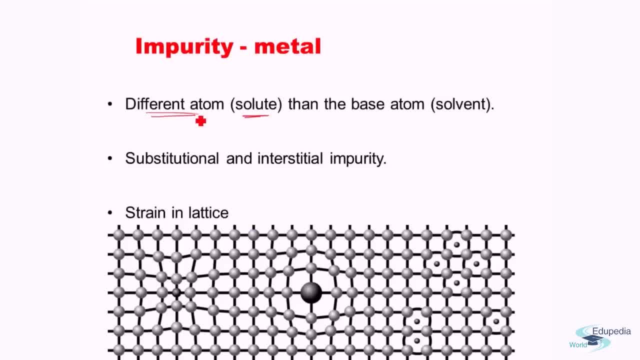 solute atom, that is, the different atom, is called solute. the base atom is called solvent, not called. rather, we can think it parallel to the that concept. then, in the case of iron carbon, what is happening is that the carbon is going into the interstitial location because it is much. 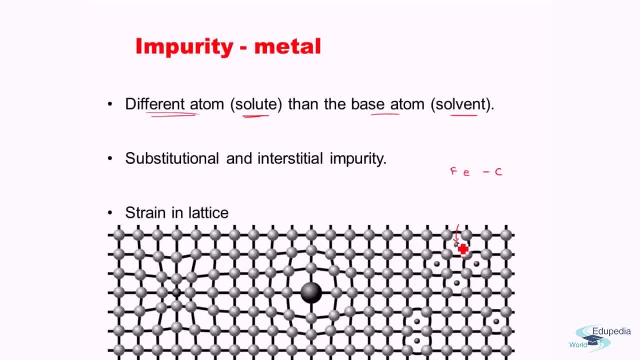 smaller. thereby we are getting interstitial impurities in the form of carbon. but since this location was supposed to be very small, then we are getting interstitial impurities, but we have added a impurity atom. this will cause distortion in the surrounding atoms. that is the 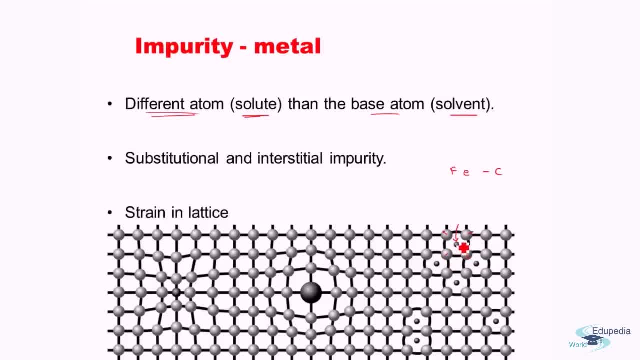 atoms will slightly move away from its original location and thereby an increase in internal energy will take place. over here, distortion energy will be created. fine, so this is what is known as known as interstitial impurity. alternatively, what can also happen is that the atom which we 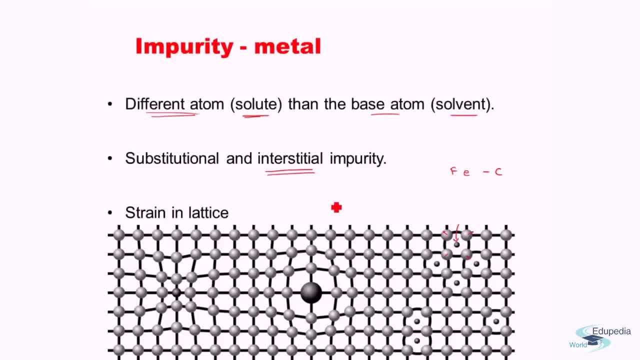 are adding is called solute. so this is what is known as interstitial impurity. adding can be quite close in size to the base atom, right? so if the base atom and the solute atom are very close in size, then instead of interstitial impurity we will get what is known as. 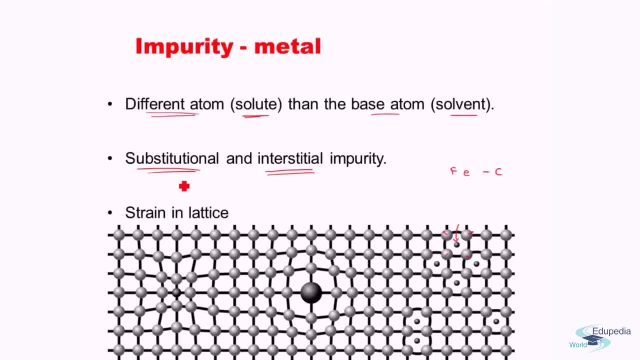 substitutional impurity. substitutional impurity will be when the base atom will be missing and in place of that the solute atom will be there. you, if the that can be in two kind of scenarios: the addition atom which is added, that is, the impurity. 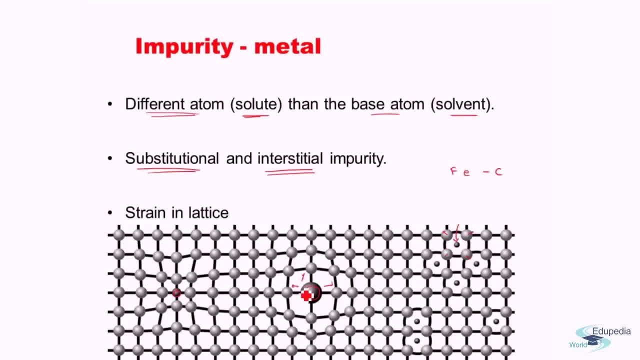 can be larger than the base atom, or it can be smaller than the base atom but similar in size. if it is larger, then it will push away the rest of the surrounding atoms to accommodate itself. if it is smaller- smaller, then it will pull the rest of the atoms towards itself in order to 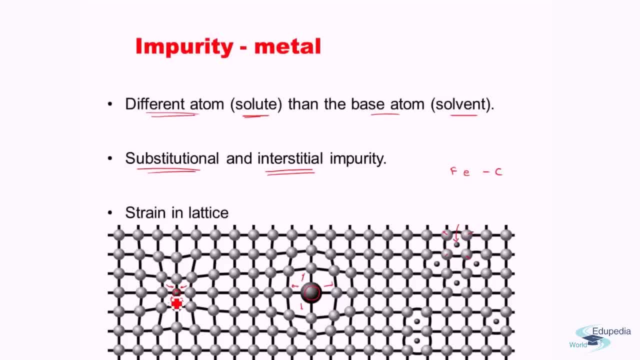 accommodate itself right. so these both cases also brings distortion in the system. but this both cases are when the atom is substituting the base atom. the impurity atom is substituting the base atom, whereas in substitute interstitial impurity the impurity atom went in the interstitial. interstitial did not. 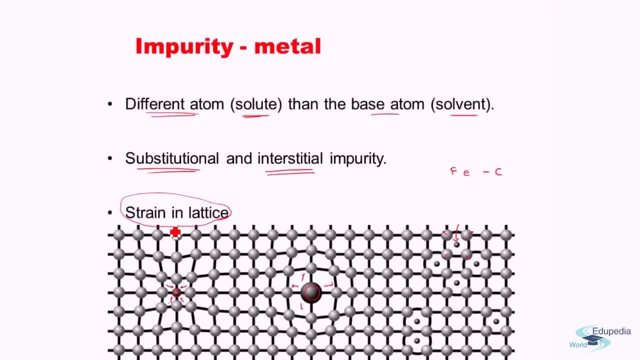 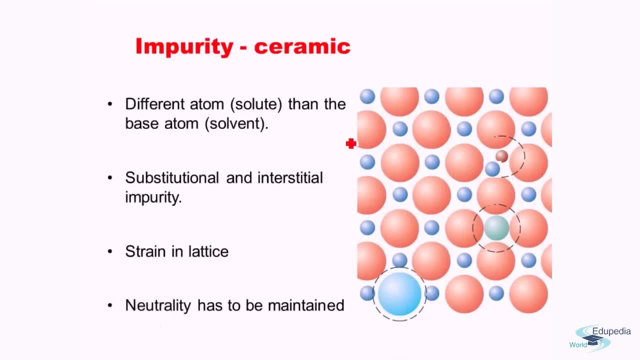 substitute and there, as I discussed, there will be stress and strain in the lattice. next, let us discuss the same concept for ceramics. this was for atom, where we see the base are the same atoms, the impurity is just additional atom, whereas in ceramics, what will happen? the base will be two or more different kind. 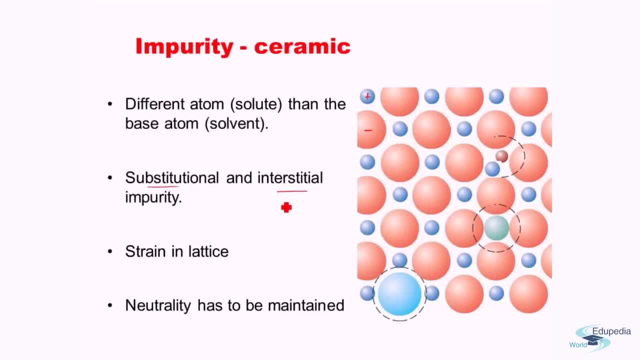 of atoms, the anion and the cation, right and here what will happen is same concept for ceramics. this was for atom, where we see the base and the, Similar to the case of metal. we can have substitutional as well as interstitial impurity. The interstitial impurity is over here, right. 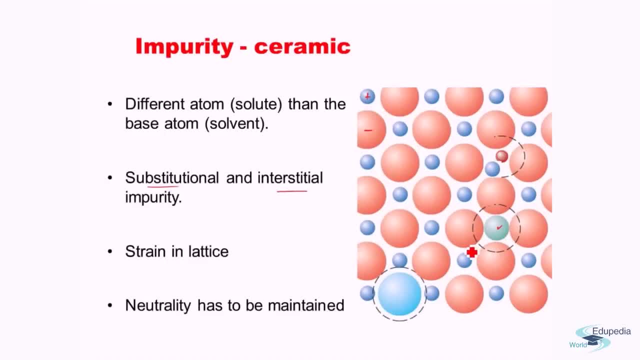 If the impurity atom is much smaller in size, then it can go into the interstitial location. If the atom is comparable to the cation, then it can substitute a cation. If the impurity atom is comparable to the anion, then it can substitute the anion atom. 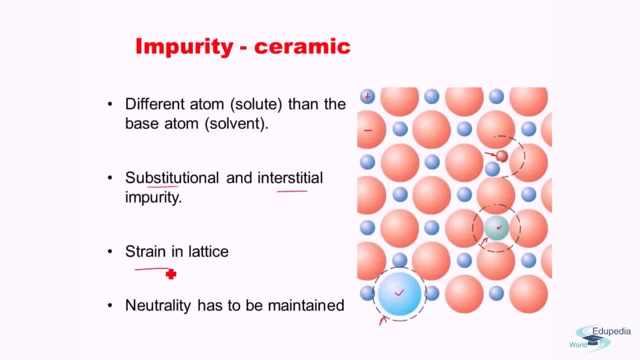 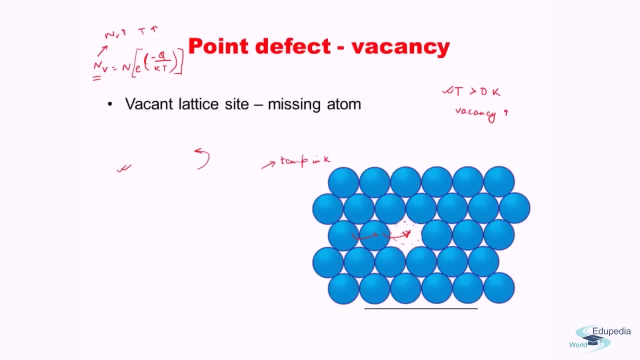 So we have the interstitial impurity, we have cationic substitution and we have anionic substitution. Similar to the case of metal impurities, ceramic impurities also produces a lot of strain in the lattice And obviously neutrality needs to be maintained in all the cases. 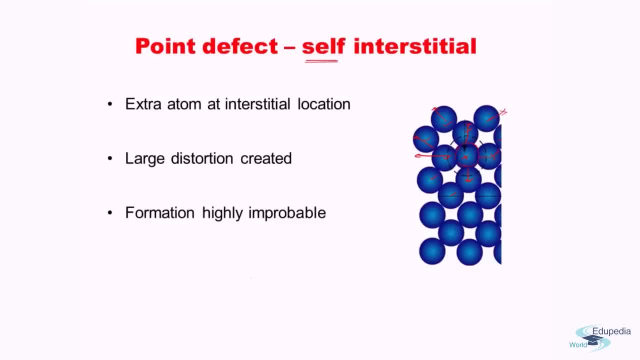 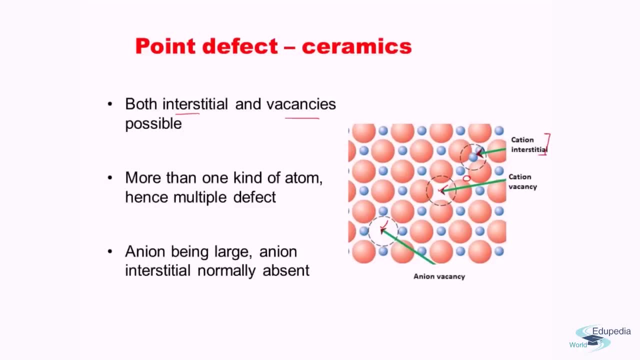 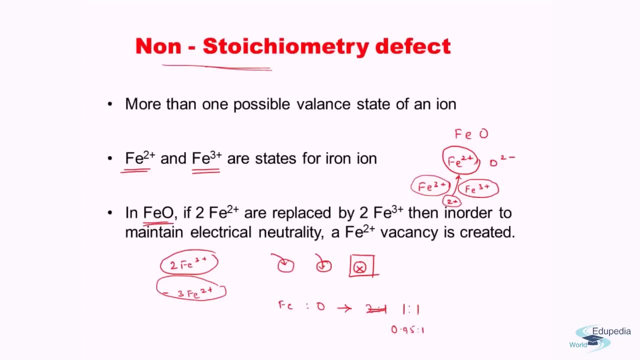 So what we discussed today was the different kind of point defects and we saw, starting with point defect as vacancy. we understood the concept. Then we saw point defects in self-interstitials, Then we saw point defect in ceramics, that is, cationic vacancy, anionic vacancy.